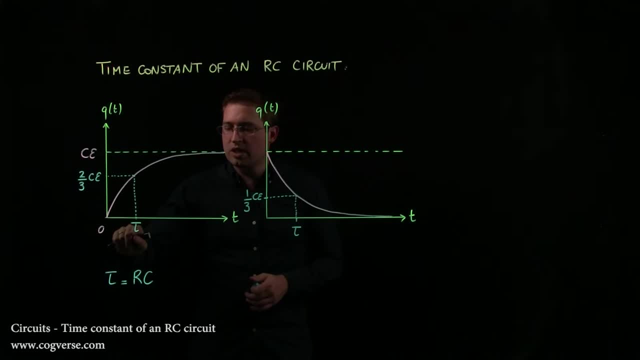 So in this case, when t equals tau, the capacitor is charged 2 thirds of the way or 66.7%, And here it's discharged 2 thirds of the way or 66.7%. And in case you ever want to find tau, if you're given a graph and you want to find, 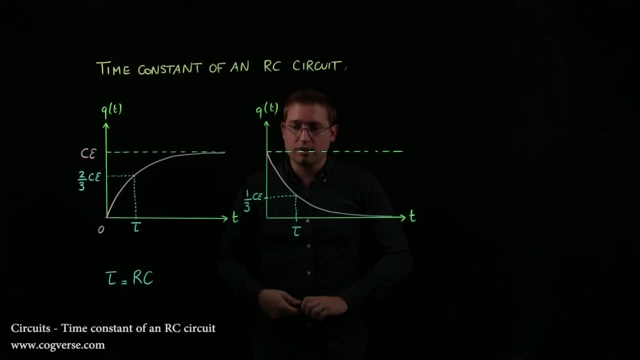 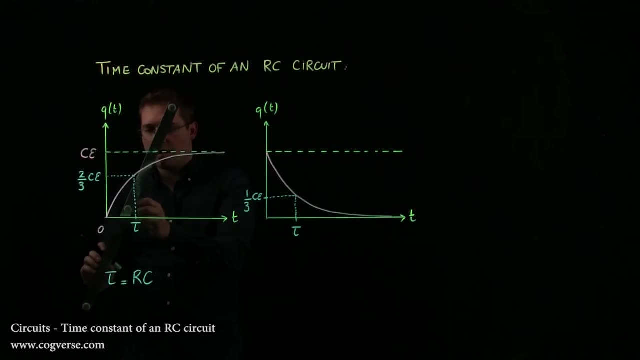 the value of tau. maybe you don't know R or you don't know C? well, there is a way to do that. You can graphically do it. All you have to do is draw the tangent at the origin And 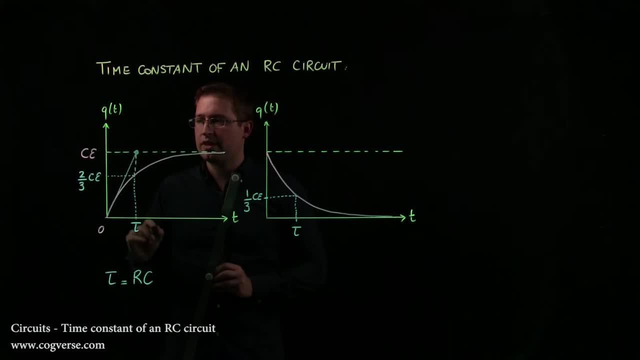 the x coordinate of the point here where it intersects with the horizontal line, equal to C epsilon. the x coordinate is equal to tau. So that's one way to get it, And of course you can do the same thing here. 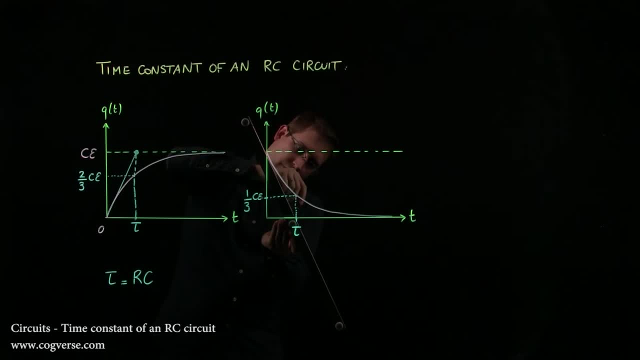 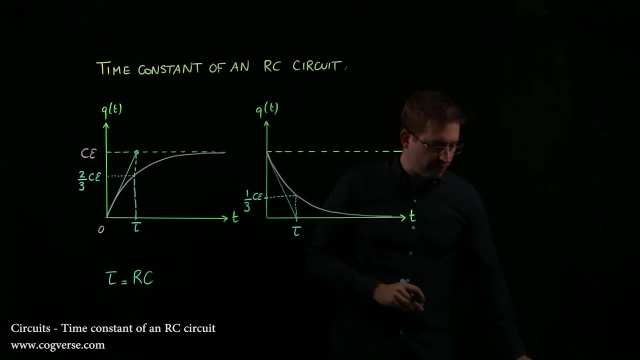 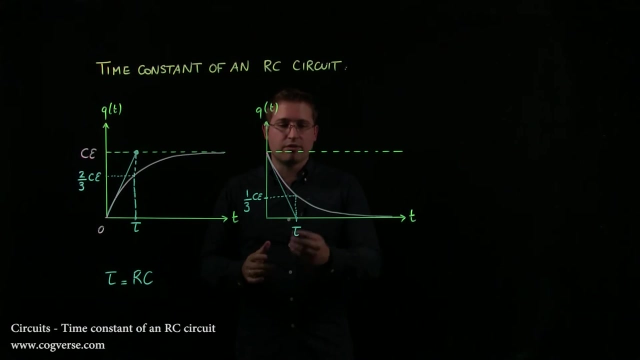 You just draw the tangent to the curve and when it crosses the t axis, that's your value of tau. So, in case you ever needed to, you could graphically derive tau from this graph or this graph. 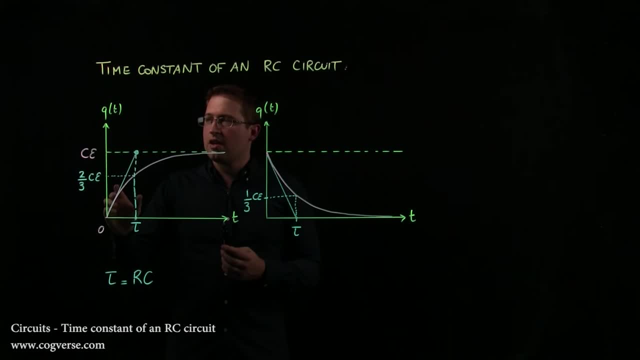 One last thing: you notice that eventually the charge maxes out at C epsilon or eventually the charge is basically zero if the capacitor is discharging. How long do you have to wait for this point? You know how long does it take to get to this point. 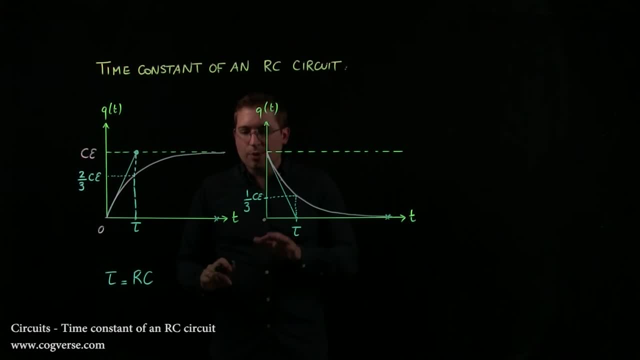 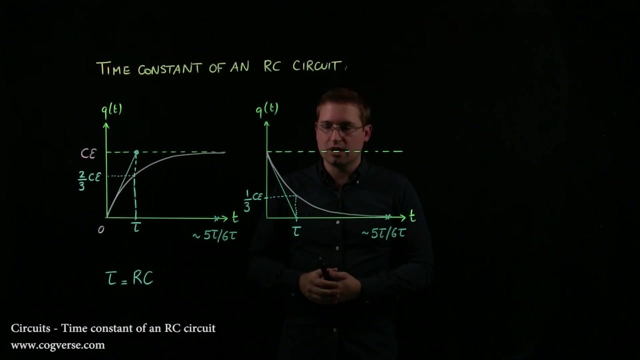 Or to this point: Well, between 5 tau and 6 tau gets you pretty close. So if your time constant tau is, I don't know, 3 seconds, you know. if you wait 15 seconds or 18 seconds, let's just say 20 to be conservative. 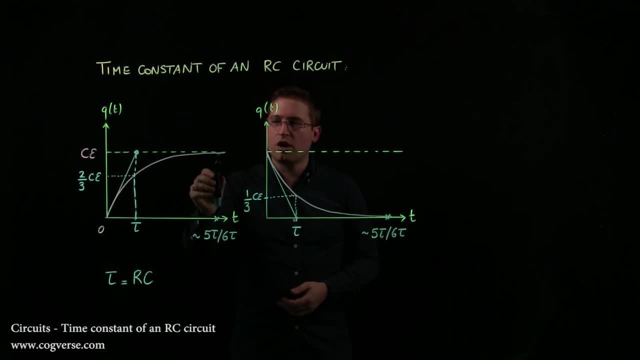 then you're pretty much here. So it's either almost very close to fully charged or very close to fully discharged, And if you want to be safe, you just take 10 tau experimentally and then you should be fine.